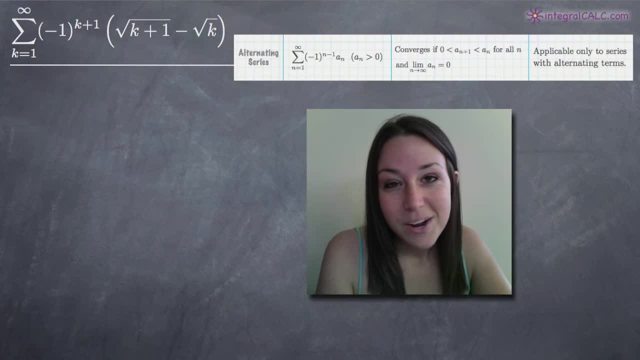 Hi everyone, Welcome back to integralcalccom. Today we're going to be talking about how to use the alternating series test to determine whether or not an alternating series converges, And in this particular case we have the sum of the series, negative one to the k, plus one. 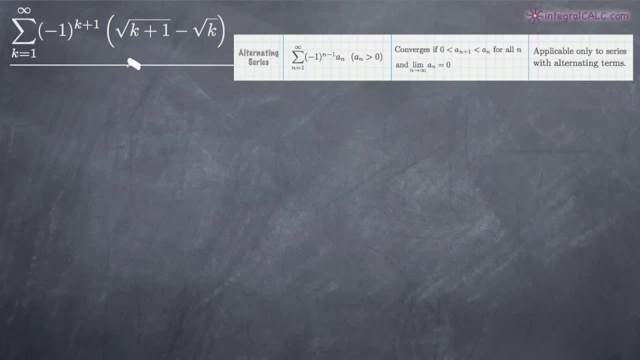 times the square root of k plus one minus the square root of k, And we've been asked to determine whether or not this series, from k equals one to infinity converges or not. So because we have an alternating series, we're going to be using the alternating series. 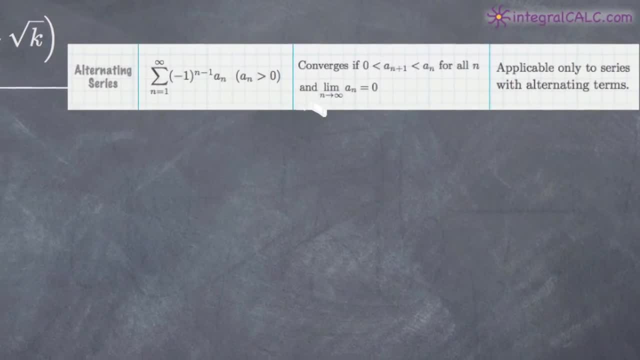 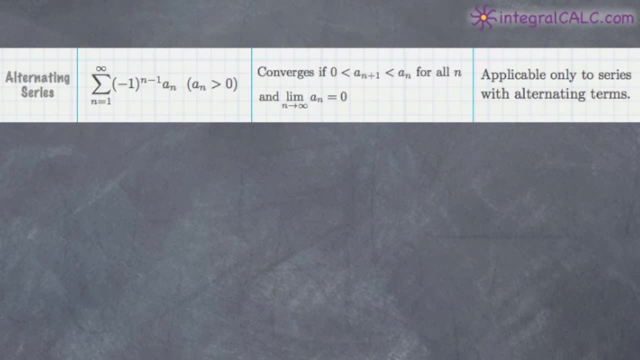 test for convergence, And I've taken here a screenshot of the part of the convergence test chart that I have up on my website that talks about the alternating series test. So what we see here is that, in order to conclude that an alternating series converges, we have 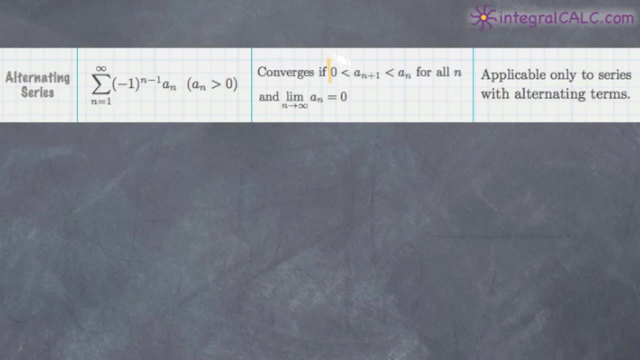 to show two things. One, we need to show that the series a sub n is always greater than the series a sub n plus one, which is also always greater than zero. And we need to show that the limit, as n approaches infinity, of the series a sub n is equal to zero. So those 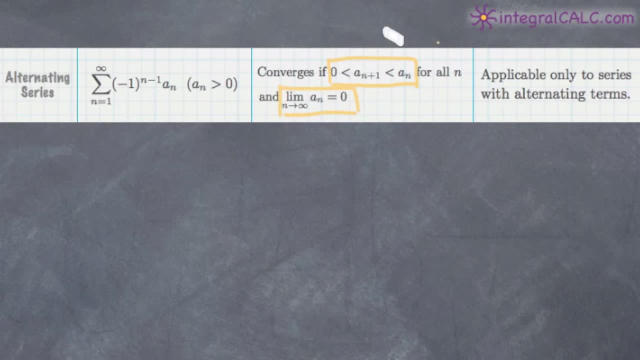 are going to be the two things that we need to do, And I'll call them one and two. So we'll start with the first piece, piece number one, where we need to show that the series a sub n is greater than the series a sub n plus one which is greater than zero. 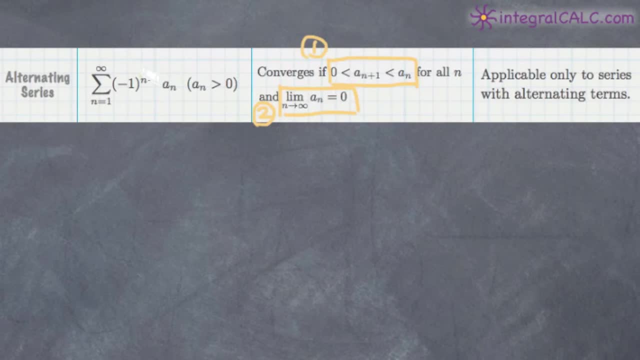 Notice here that the series- a sub n- is always greater than the series a sub n plus one, which is equal to zero. Notice here that in our formula right for the alternating series, we have here a sub n, We've got a sub n, and then we also have this piece here. 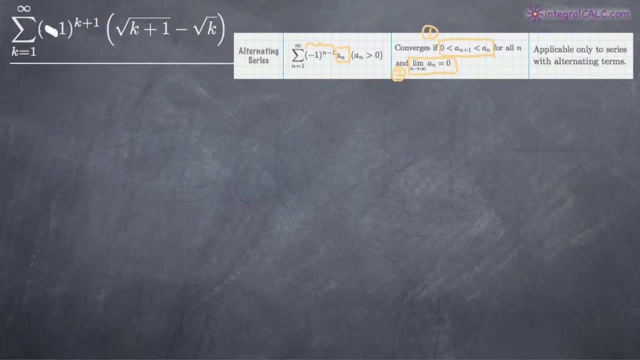 which is the alternating series part of the series. What this tells us is that our series is divided into two pieces: The first part, which gives us the alternating series part, and that's going to be the negative one raised to some exponent, whether or not it's k or. 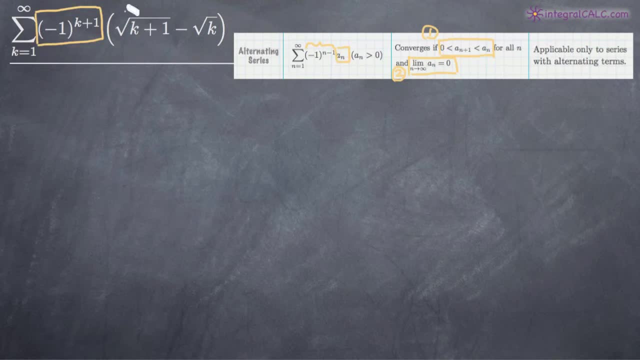 k minus one or k plus one. That's the alternating series part And the second part here. everything after that is going to be our series, a sub n. So this second part right here is going to be a sub n. So we'll use that as a sub n We. 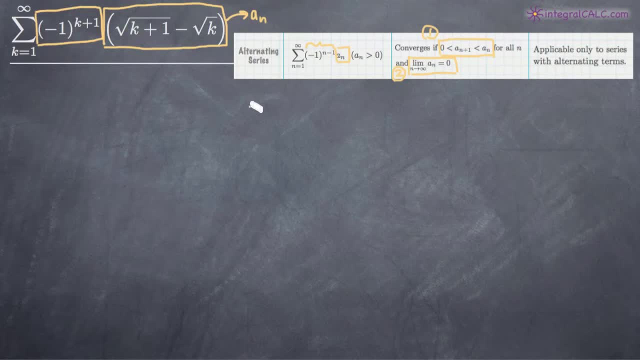 need to show that that series, a sub n, is larger than the series a sub n plus one. So I'm going to show you two ways to do that. The first is kind of just to get an idea in your head of whether or not it is greater. The second is prove that it's greater. 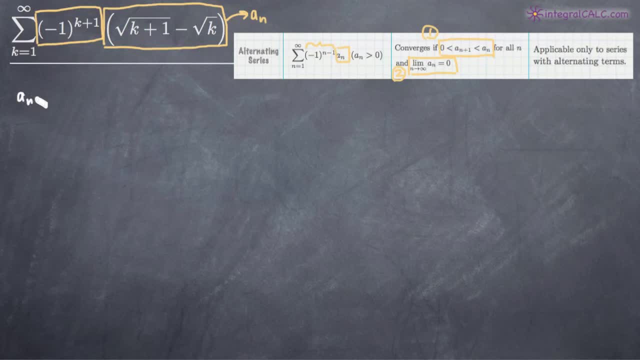 So the first way I'm going to show you is we'll say that the series a sub n is equal to the square root of k plus one minus the square root of k. So we have that as the a sub n series. If we start plugging in for k and we start with one, because they tell 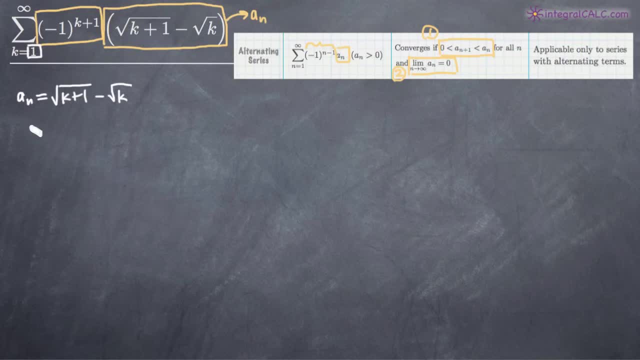 us. we're starting with one here. If we start plugging in and let's see, we'll get one, two, three, four. We'll just plug in four terms. If we plug in one, we'll get the square root of. we plug it in here and here We'll get the square root of two minus the square. 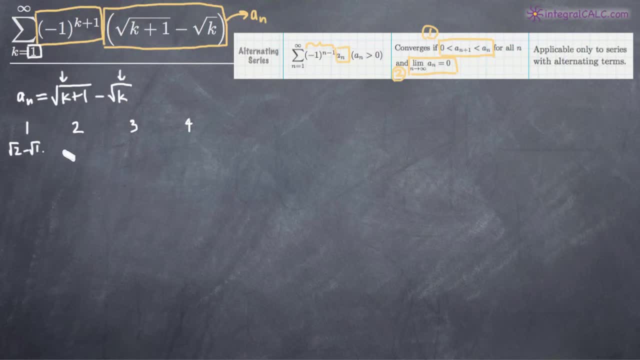 root of one. Then if we plug in two, we'll get the square root of three minus the square root of two. Then when we plug in three, we'll get the square root of four minus the square root of three And, as you can see here, the square root of three minus the square root. 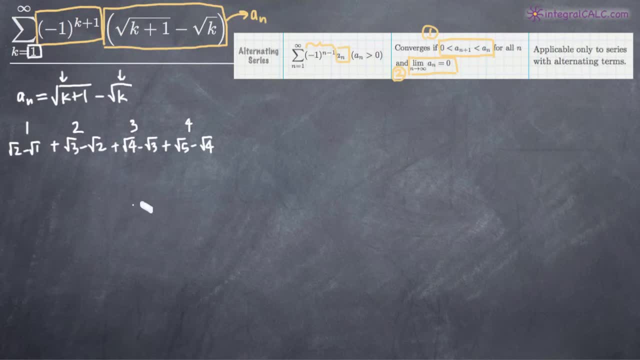 of four. So those are going to be the terms we're going to get when we plug in one, two, three and four on into infinity. We'll get these terms here to repeat. So we'll plug those values in for k. Then, if we look at a sub n plus one, the first thing that we 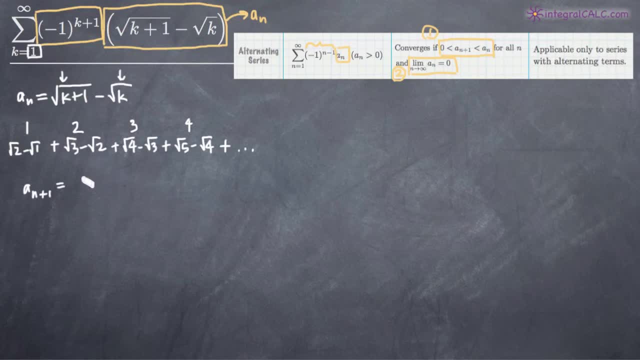 can try is just to replace k with k plus one. So we'll say k plus one is equal to a sub n plus one. So k plus one is going to go in for k right here. So then we'll have another plus one And then we're going to plug in k plus one here for the second k. So when 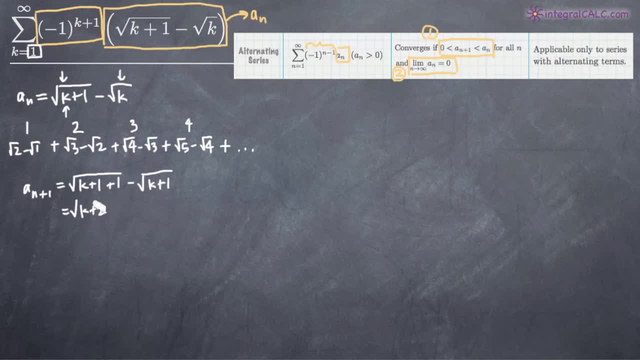 we do that, obviously we get the square root of k plus two minus the square root of k plus one. So when we do that, if we plug in again one, two, three and four, we'll get starting with one, two, three and four plus one. We'll get starting with one, two, three and four. 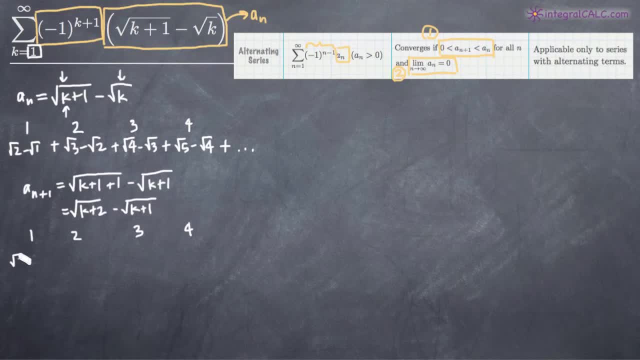 root of 3 minus the square root of 2, plus the square root of 4, minus the square root of 3, when we plug in 2 plus the square root of 5 minus the square root of 4, which is what we get when we plug in 3, and then obviously the square root of 6 minus the square root. 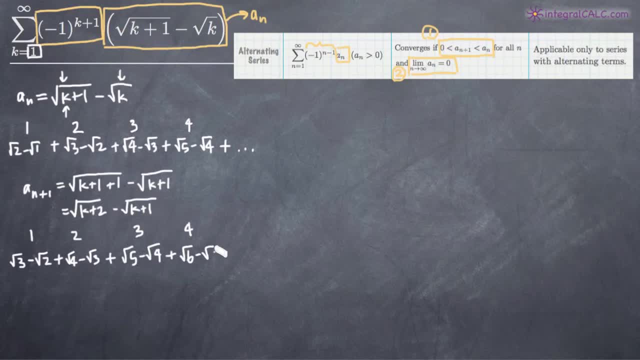 of 5 when we plug in 4.. What we can see is that if we compare this first term here, if we compare the square root of 2 minus the square root of 1 to the square root of 3 minus the square root of, 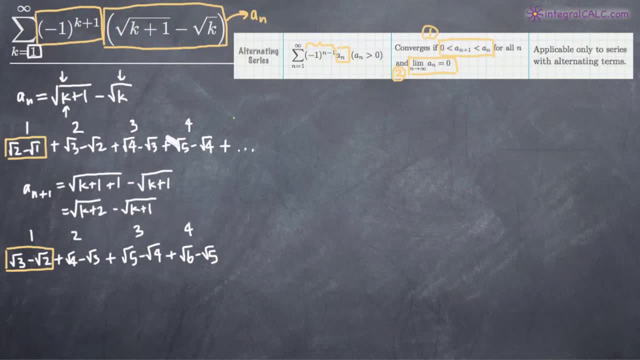 2 and then we compare every term in the series. right, When we plug in 2, we got this term and we got this term. When we compare each one of those terms in the series, what we find is that a sub n. 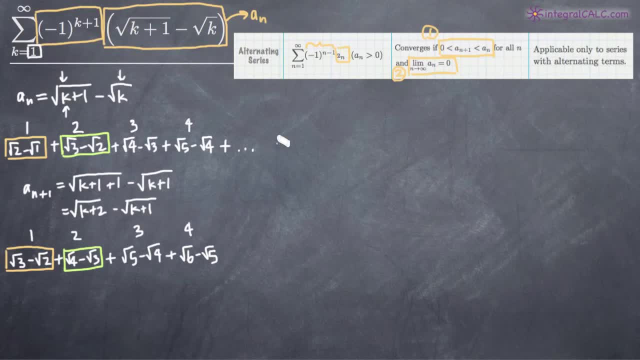 these terms up here are always greater than the a sub n plus 1 terms, So we conclude that a sub n is greater than a sub n plus 1.. Okay, So that's what we get when we plug in k plus 1 for k, which is what we want up here, right? 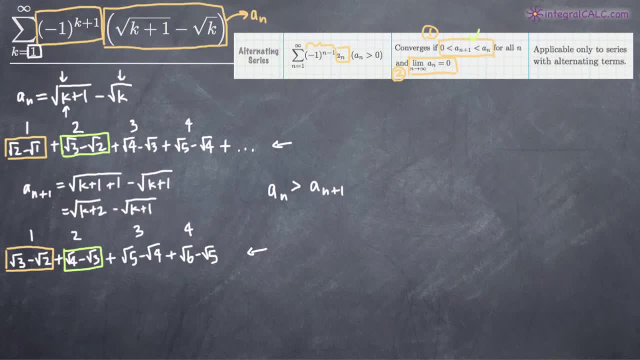 We want a sub n to be greater than a sub n plus 1.. So that's how we can kind of get an intuitive gut feel that this is going to work. But what we want to do is prove that a sub n is greater than a sub n plus 1.. 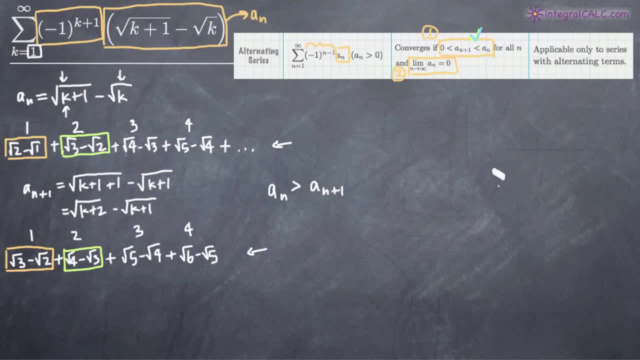 And the way that we can prove it is by taking the derivative of a sub n, the series of n plus 1.. If we take the derivative, it's going to tell us whether or not our series is increasing or decreasing. And if the series, if we can show that the series, the derivative, is negative, the series 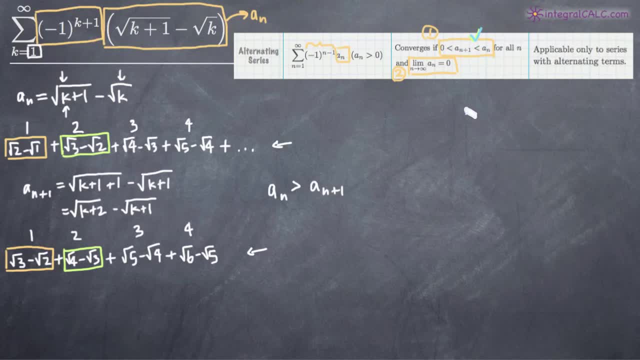 is always decreasing, then of course, a sub n plus 1, a term further along in the series- will always be less than a sub n, which is what we want to show. So I'll go ahead and show you that now. If you take the derivative of a sub n, we'll say that a sub n plus 1 is greater than a. 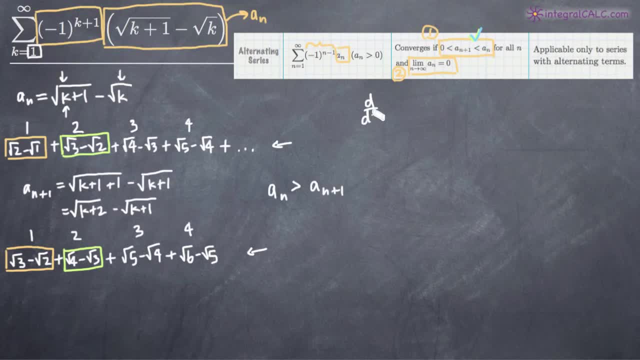 sub n plus 1.. We'll say d dx of a sub n. the derivative of a sub n is going to be: and let's go ahead and transform this here into k plus 1 to the 1 half minus k to the 1 half, which is the. 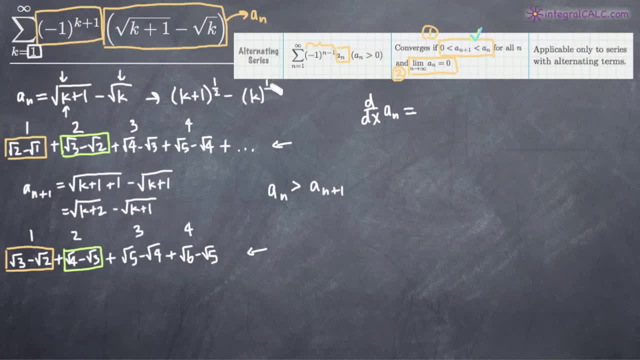 same thing as keeping the square roots in there right. The square root is the same thing as taking what's under the square root and raising it to the 1 half power. So when we take the derivative we'll multiply that 1 half out in front. 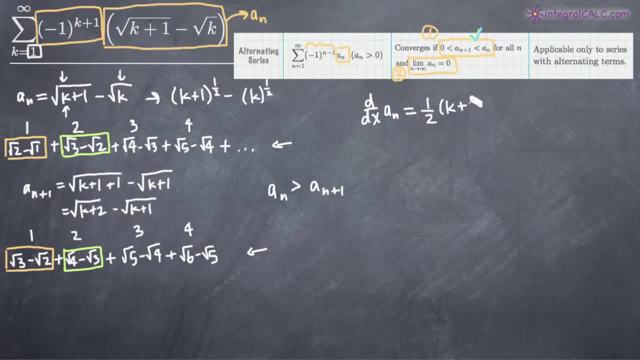 We'll take the derivative. We'll take the 1 half out in front, k plus 1 to the negative 1 half, and then we'll get minus 1 half times k to the negative 1 half. So when we simplify this we'll end up with 1 over 2 times the square root of k plus 1,. 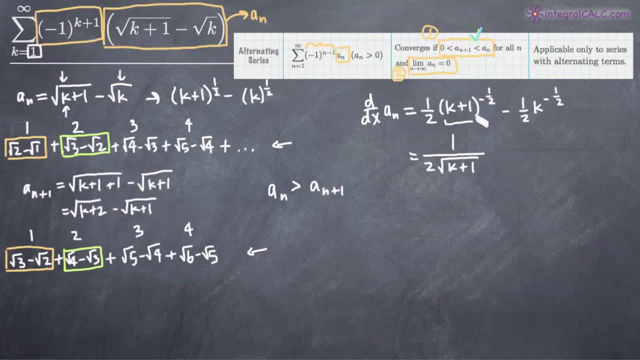 which we get because we move this whole term here, k plus 1, to the negative 1 half. we move that to the denominator to make the 1 half exponent positive. when we move it from the numerator to the denominator The exponent becomes positive and then of course we're back at positive 1 half, which. 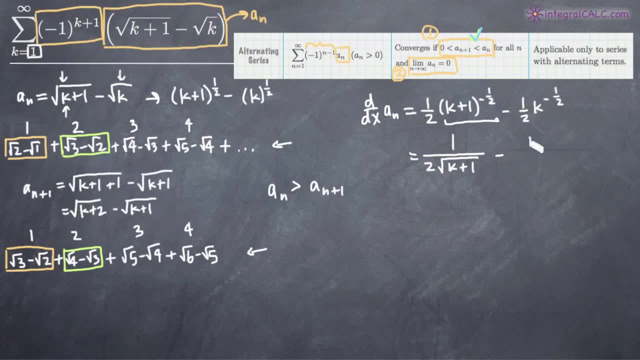 is the same thing as the square root. So then, similarly, over here we've got 1 over 2 times the square root of k. Now if we want to find a common denominator here, we would just go ahead and multiply this first term times the square root of k over the square root of k, and we'd multiply. 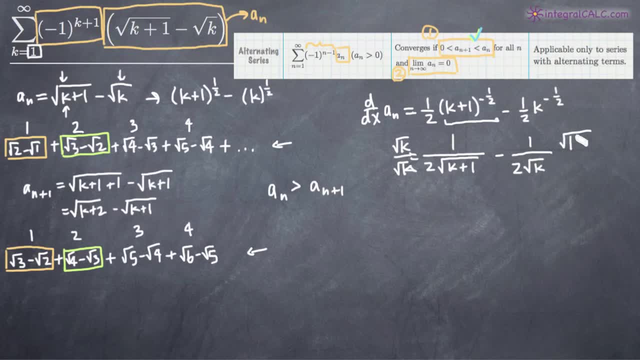 the second here by the square root of k plus 1 over the square root of k. When we simplify this, we'll end up with the square root of k minus the square root of k plus 1, all over 2 times the square root of k, times the square root of k plus 1.. 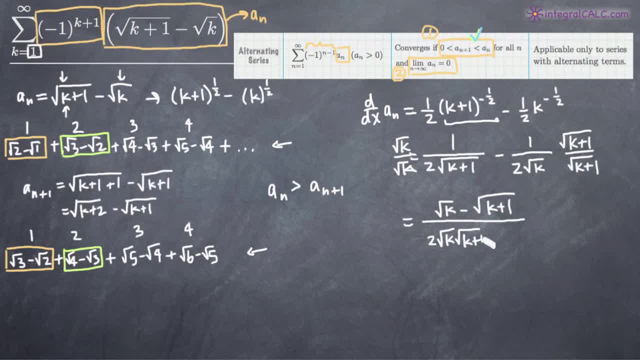 2 times the square root of k. yup. So now to simplify further, what we can do is go ahead and multiply by the square root of k. Remember, from limits we can multiply by the conjugate of the numerator. here It's the same two terms, but instead of the negative sign in between them, we put a positive. 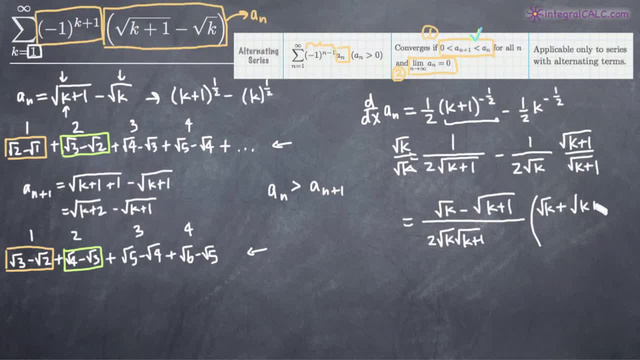 sign This term right. here is the conjugate of the term from our original numerator, So k plus k plus 1, we multiply the numerator and the denominator by the conjugate, so that it's the same thing as multiplying by 1.. And when we now multiply these out, we multiply the denominator by the conjugate. 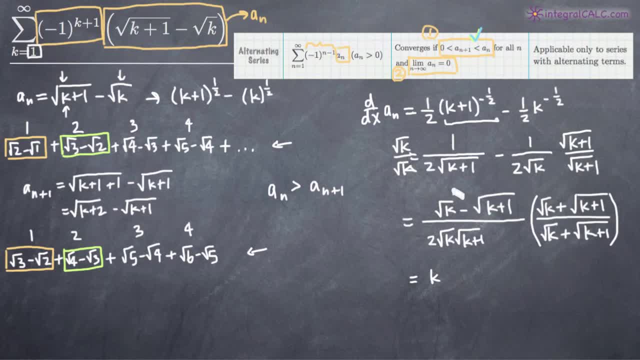 So when we multiply these out, we'll get k right This times. this gives us k, and then we have plus the square root of k times the square root of k plus 1, minus the square root of k times the square root of k plus 1.. 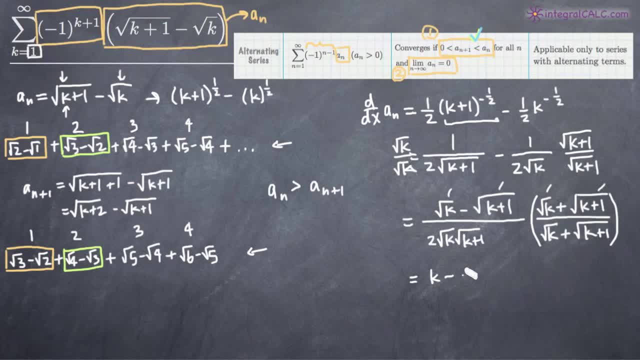 So that cancels, and then when we multiply these two terms together we're just left with minus k plus 1. So we get that together and then in the denominator here we'll have: and let's combine these two terms. You can combine those by putting everything underneath the square root sign. when two square 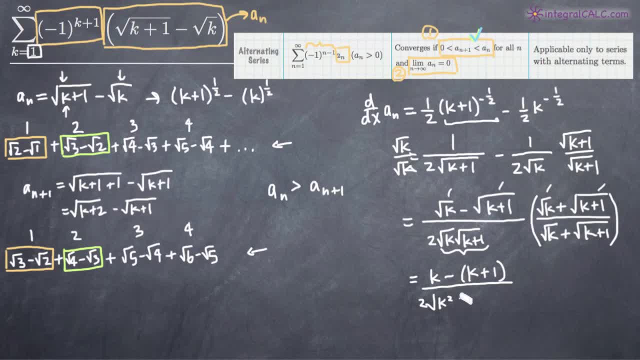 roots are multiplied together. So we'll just do: k squared plus k will be underneath the square root sign there, and then we have times: the square root of k plus the square root of k plus 1.. So now you can see that we've got a k and a minus k, so these two are going to cancel. 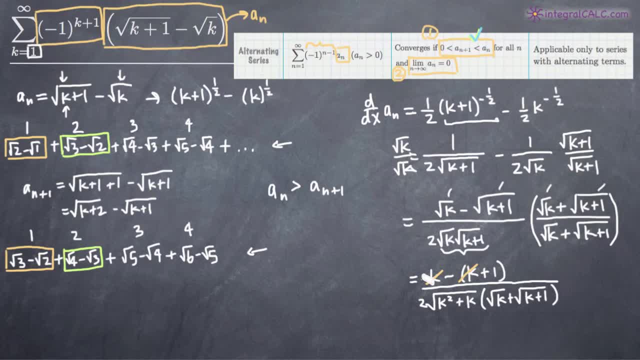 and all we're left with here. Okay, And let me just go ahead and cancel out this whole thing. All we're left with in the numerator is a negative 1.. So this is our derivative right d dx of a sub n. 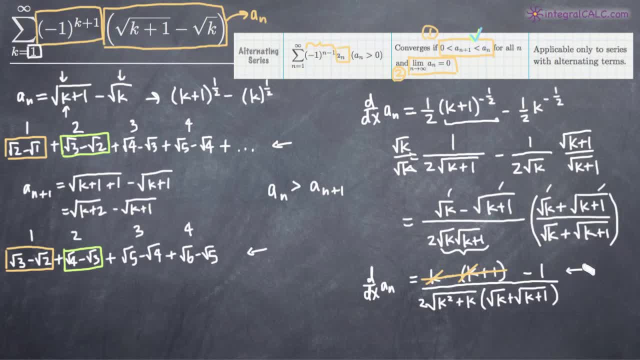 This is our derivative, and what you can see is that the numerator is always going to be negative. right, It's a negative 1.. The denominator is always going to be positive because our series starts with k equals 1, right, We start with 1.. 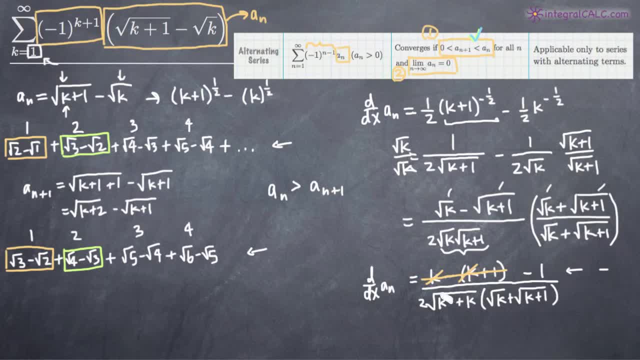 If you plug in 1 or any number, A number larger than 1 in for k, into our denominator here, obviously you're going to get positive 2 there. You're going to get positive underneath the square root sign here, right, Because you'll get a positive number squared plus another positive number is always going. 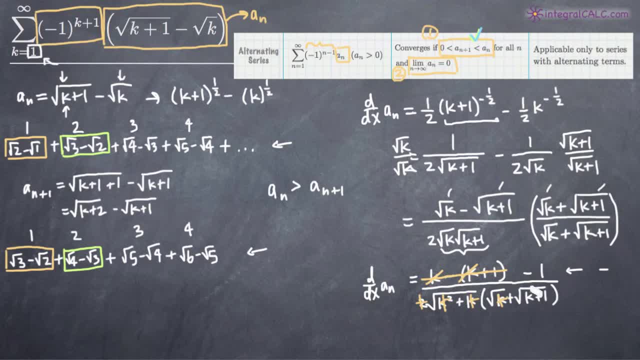 to give you a positive number underneath that square root sign: positive and positive again. So everything in the denominator is positive. So since you've got a negative divided by a positive, that's always going to be a negative, which means that the derivative d dx of a sub n is always going to be negative, and so it's. 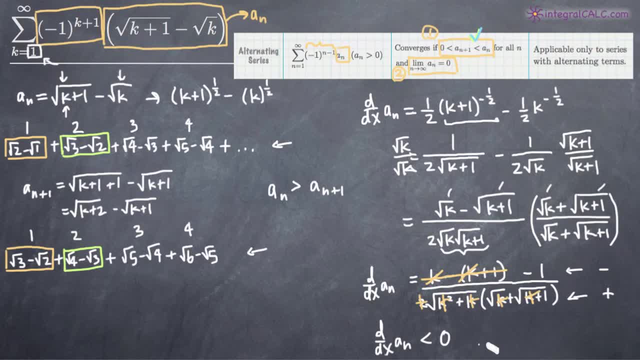 always going to be less than 0, which means that the function is always decreasing. So the function is always decreasing, right? Our series basically goes: a sub n plus a sub n plus 1 plus a sub n plus 2, plus dot, dot, dot, right. 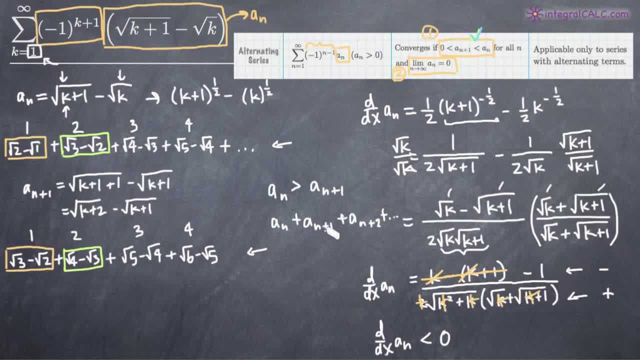 Since the series is always decreasing, This will always be. a sub n plus 1 will always be less than a sub n. a sub n plus 2 will always be less than a sub n plus 1, and the series will be constantly decreasing. 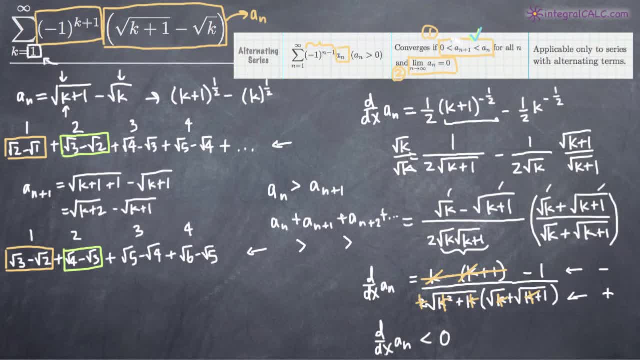 So we've now proven here that a sub n is greater always than a sub n plus 1.. We also know that a sub n plus 1 is always going to be greater than 0, and we can see that over here in our denominator. 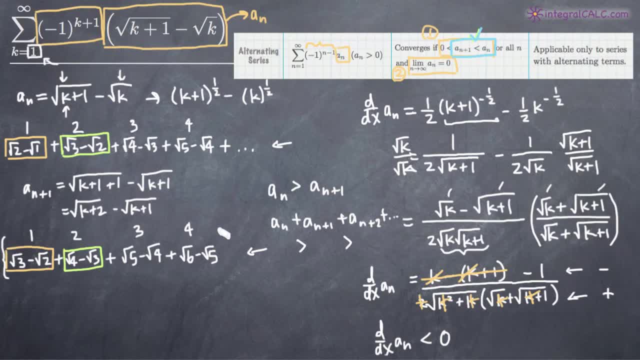 In our series that we've written out these terms right here. right, No matter how large you go, right, 400 terms out or whatever, you're going to have the square root of 400 minus the square root of 399.. 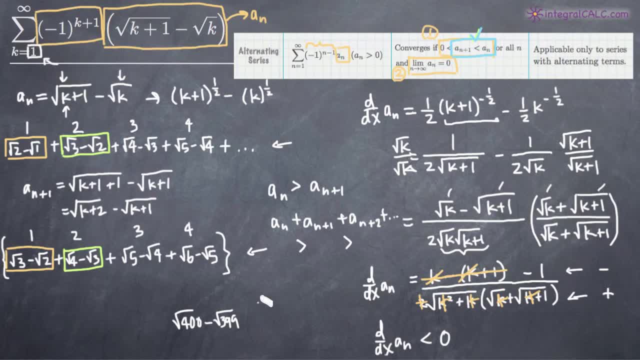 That's always still going to give you a positive number. It will always be positive and therefore always be greater than 0.. So we have now officially checked off these two requirements right. We've proven there that a sub n will always be greater than 0.. 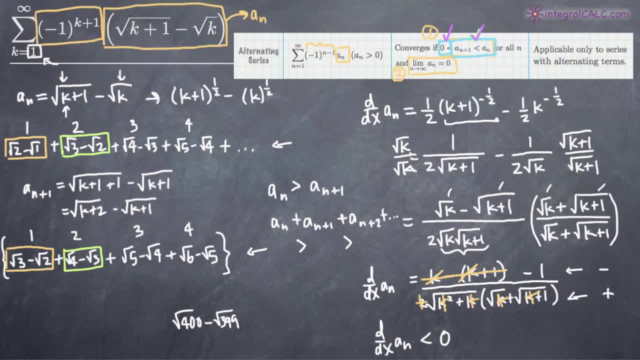 It will always be greater than a sub n plus 1, which will always be greater than 0.. So that's how you can prove, using the derivative, that you've met that first requirement. So now all we need to do is determine whether or not the limit of a sub n as n goes to infinity. 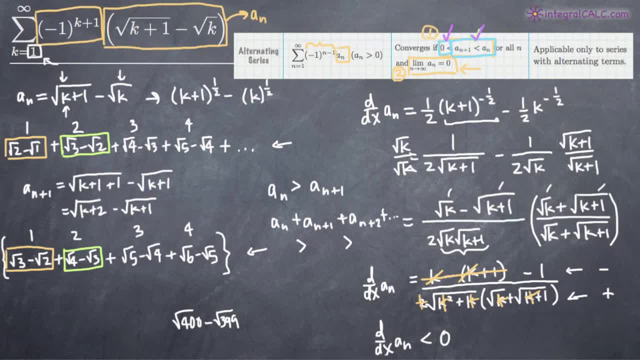 is equal to 0, number 2.. If we can prove that, then we know that this series converges. So let's go ahead and look at that. I'm going to just erase this stuff here, so I've got some more room. 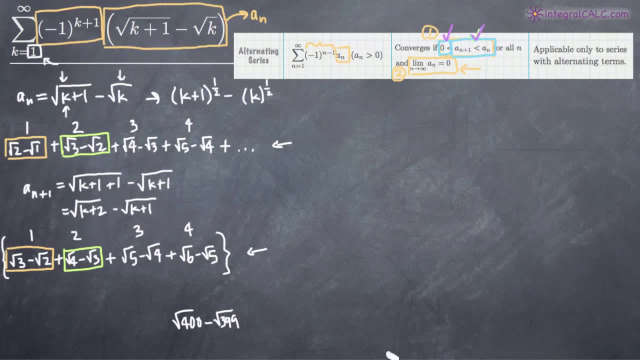 So to show that the limit is equal to 0,, what we'll go ahead and do is take the series a sub n. So remember that the series is the square root of k plus 1 minus the square root of k. This series up here, this is a sub n. 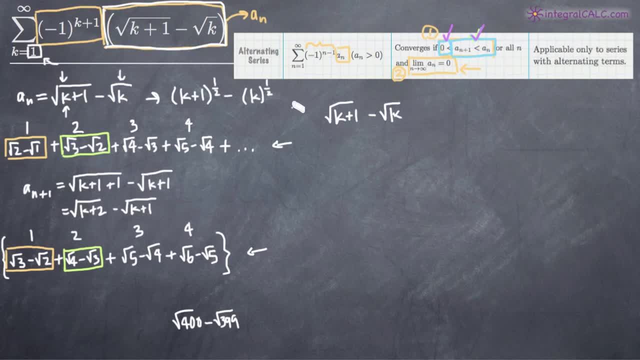 And what we want to do is find the limit of this series. Okay, So we want to find the limit of this series as n approaches infinity And we want it to be equal to 0.. We can see roughly, just by looking at it, that it's probably going to be equal to 0. 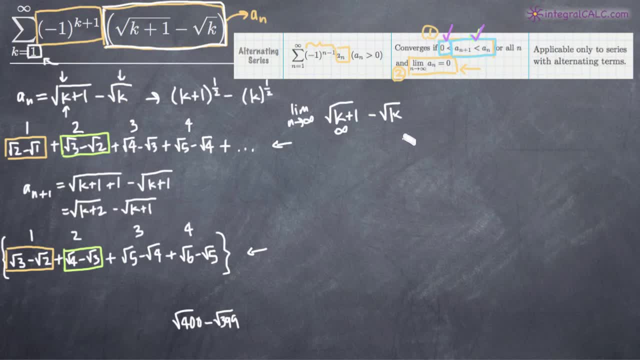 If we plug in infinity for k right here, we'll get infinity plus 1, which 1 compared to infinity is nothing, So it's basically infinity. And then we get infinity here. Square root of infinity minus square root of infinity should be 0.. 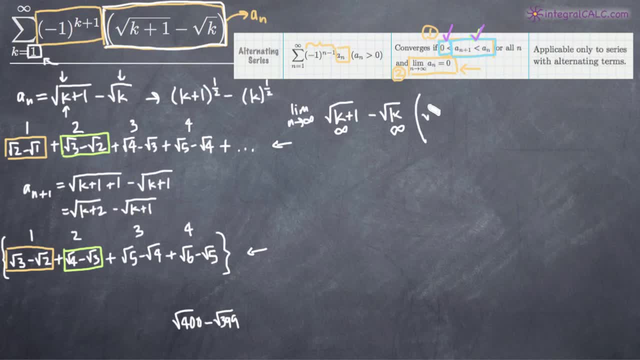 But the way that we can prove this is by multiplying again by the conjugate, And that will allow us to see very clearly that the limit is going to be 0 as k approaches infinity. So we'll multiply by the conjugate, which is square root of k plus 1 plus square root. 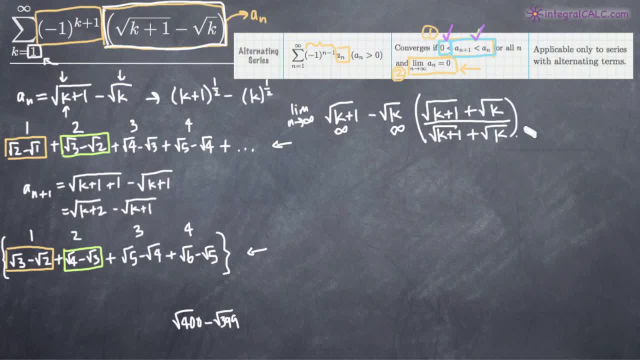 of k. So when we multiply by the conjugate, we'll see that we'll get k plus 1.. Then we'll have plus square root of k times square root of k plus 1, minus square root of k times square root of k plus 1.. 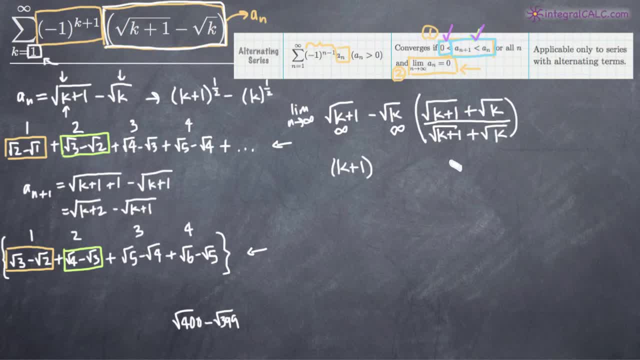 Which will cancel each other out, And then we'll just be left with, when we multiply this one by this one, a minus k. So that will be our numerator, And then in our denominator we'll end up with square root of k plus 1 plus square root. 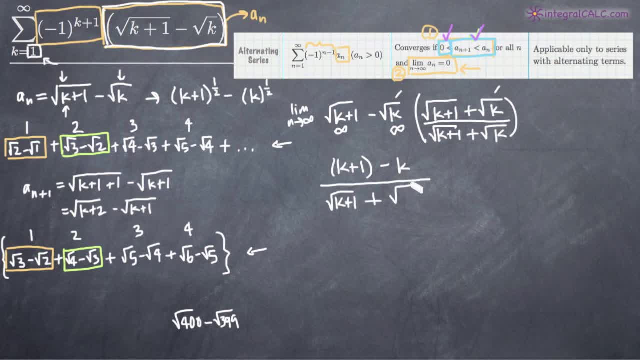 of k And we want to be finding, of course, the limit, as k goes to infinity. So we can see, obviously, that k and k plus 1 are equal to infinity. So we'll be left with 1 over the square root of k plus 1 plus the square root of k. 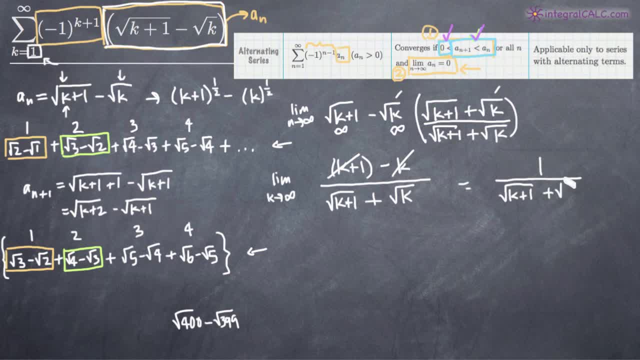 And this should make things very clear for us, because obviously our denominator now, when we plug in infinity here for k, our whole denominator is going to be very, very, very large, infinitely large. And we know from doing lots of these problems that when we plug in infinity we're going.